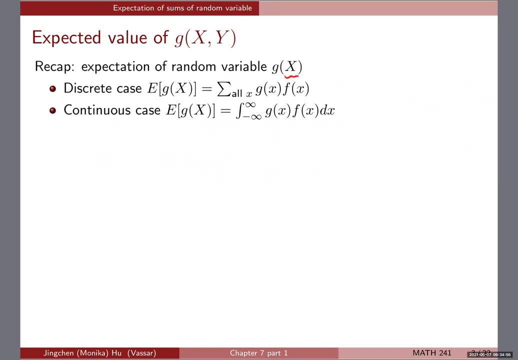 okay. so if I have like a random variable, x, right, and now if I have a function, gx, okay, then what we know that if you're working with a discrete case, you are doing a summation right of all of the possible x values of gx times, fx. where fx, or sometimes you write px. 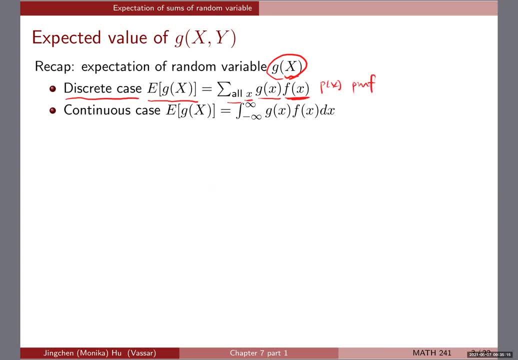 is the pmf? okay, for the discrete case, okay, And then for the continuous case, we know that the expectation of this function, gx, becomes the integral right of gx, fx, dx, where fx is the pmf pdf. sorry so let me write it down here, okay? So, depending on what type of 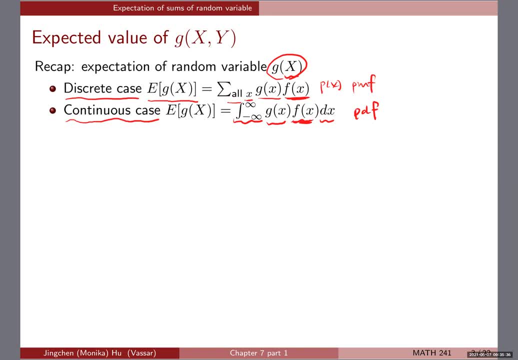 variables you're working with. you have this two different set of approaches, okay. So now suppose you have a function. okay, now is a gxy function. okay, it is a real value function of random variables, x and y at the same time. okay. So, for example, something like x plus y, x minus y, x times y, things like: 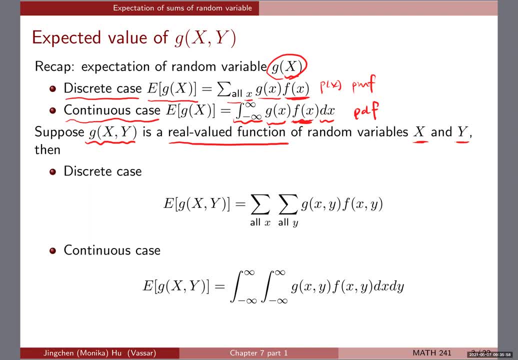 that they are right, or x squared plus y, any kind of function you can think of about x and y at the same time. it could be a gx function, okay. So for the discrete case, meaning that if I have both of them- both x and y, to be discrete- 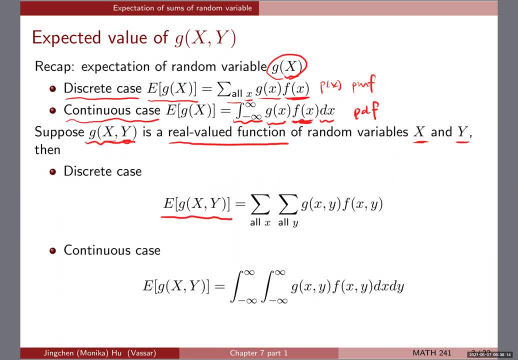 okay, then the expectation of this gxy function, as you can see, becomes a double sum. okay, because we're summing over all of x and all of y. okay, we have the gxy function, which is the function we're evaluating, multiplies with the joint. okay, so here this is the joint pmf. 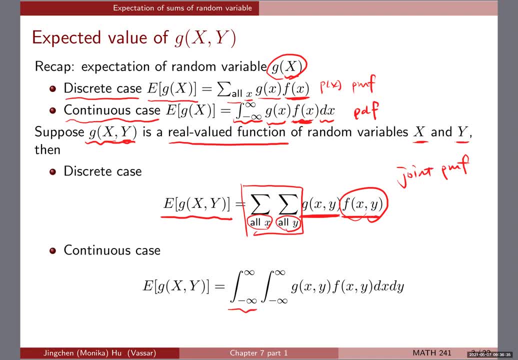 okay, And similarly for the continuous case, we're doing a double integral. okay. Now here is gxy. it's the function that we're evaluating. this is the joint pdf. okay, And then double integral. you're doing dx, dy, or maybe. 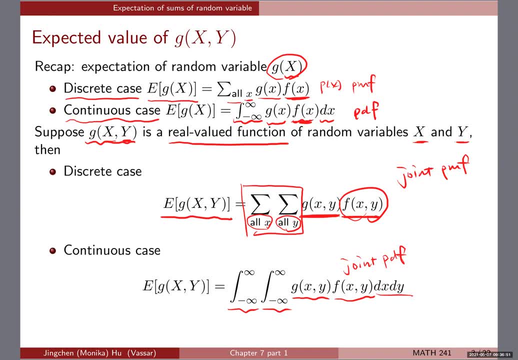 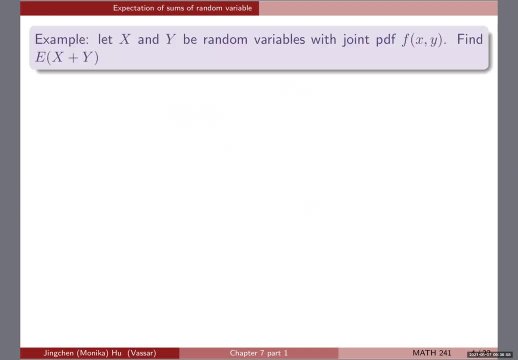 whichever is easier, you do dy, dx, okay, So try to figure out the way that works the best for the scenario. okay, So now let's look at example and a very important result: okay, So, let x and y be random variables with the joint pdf. okay, So here, as you can see, we are working with constraints. So let's look at the example and a very important result. okay, So let x and y be random variables with the joint pdf. okay. So here, as you can see, we are working with constraints. So let x and y be random variables with the joint pdf. okay. So here, as you can see, we are working with. 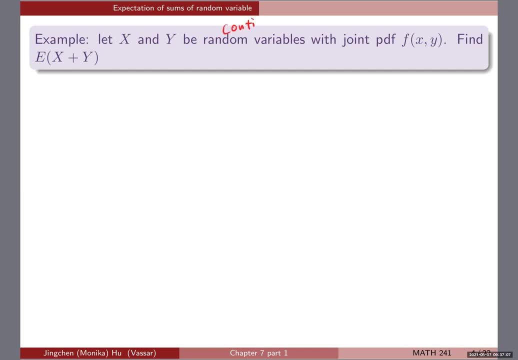 continuous, okay, And so, as you will see soon, we will be doing a double integral in this case. okay, So the joint pdf is fxy. okay, They asked you to find the expectation of the sum of the two. okay, So, following what we had from the previous slide, okay, So the g. 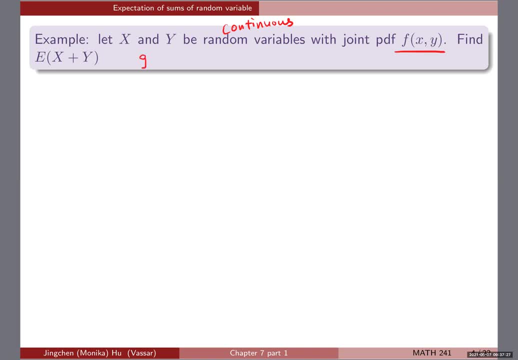 so let me write it out over here, okay, So the gxy function that we're doing, that we're dealing with over here, is the x plus y. okay, So notice that. remember earlier, the formula that we know is the expectation of g, x, y function. okay, so here we're. 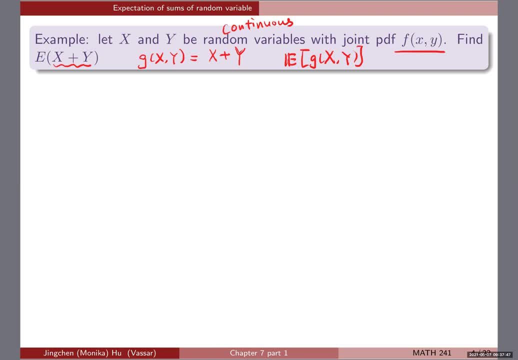 looking for expectation of x plus y. so that's another. just think about it, right, that this is a g x function, g x y function, all right, so let's get started with that, okay? so remember, what we're having is the joined pdf right multiplies with the g x y function that we're dealing with, and 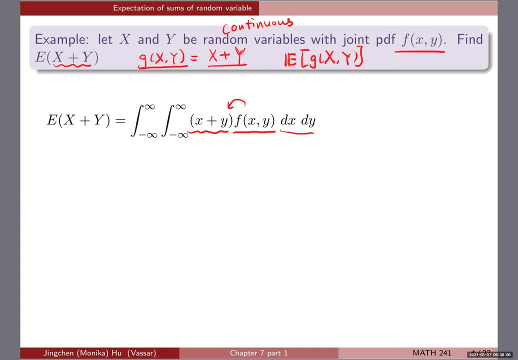 then right now i'm just writing d, x, d y, generically in a sense, and all of the bounds are from negative infinity to positive infinity. okay, so one thing: we can keep working on this. as you can see that well, it's x plus y, right multiplies with the f x, y, so i can actually break this into two parts. 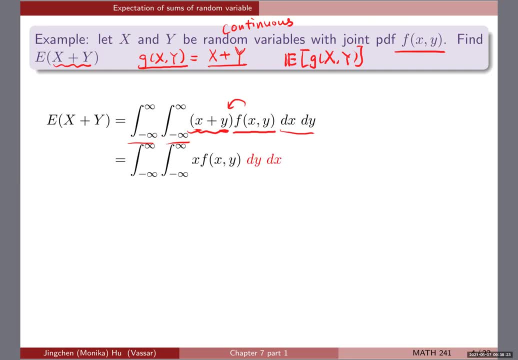 okay, the first part will be: i'm looking at the part of x times, f, x, y. okay, so i'm doing it over here. notice that i start to write d, y, d, x. you're going to see soon while i do the change, because it will be. 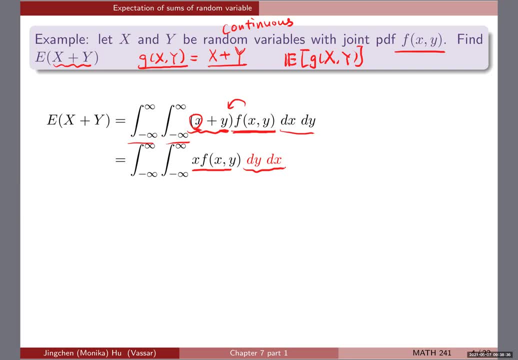 easier to do the integration um soon as you can see it, okay, and then the second part will be: uh, the y part, right, the y times, f, x, y part, and then i'm just doing d, x, d, y, because it will be easier to do um next as well. okay, so from this line to this line is purely just break x plus y times, uh. 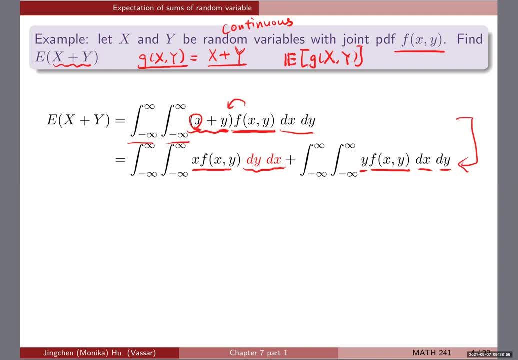 f, x, y into into two parts, and then there are two separate integrals here. okay, so now i hope you can see why i want to do like d y, d x, and then i'm just doing d x, d y, because it will be easier to do. 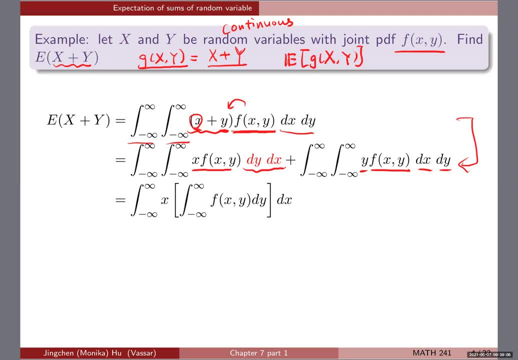 in the first place? uh, in the first case because, um, if i'm doing d, y, d x, one thing we could immediately do is that this x, okay, multiply with f, x, y. uh, this x is a constant right with respect to y, so i can bring my x outside of the first integral or the inner integral. okay, so now i have. 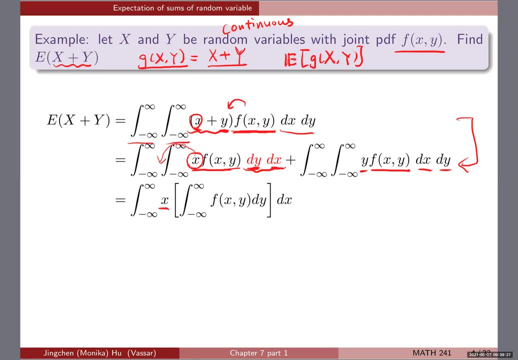 x here, and then i'm doing, uh, my integration right of f x, y, d y from that infinity to positive infinity, okay, similarly i do that. and then i'm doing f x, y, d y, and then i'm doing f x, y, d y from that for my second term, and then that's also why i'm doing d x, d y over here, because y. 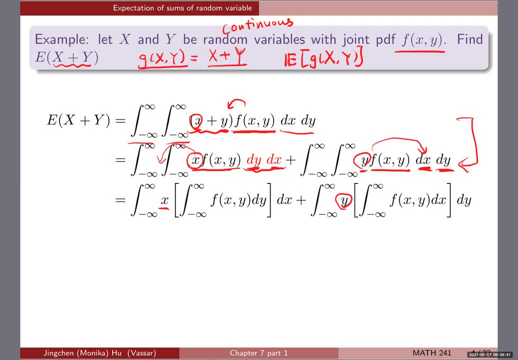 is a constant with respect to x, so i can bring it out, okay. so now, um to move forward, um notice what this is okay, so let's take a pause. this is doing a joint right integration of the joint of x and y joint pdf with respect to y, and we know that when we do that integration, this will give you. 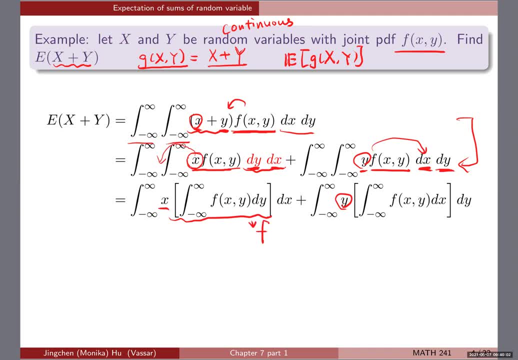 right, the marginal of x. okay, you're integrating out. so let me write it this way: okay, you're integrating out y of the joint, so you're getting the marginal of x. okay, so, similarly, you're going to get the marginal of y over here. okay, so that's. 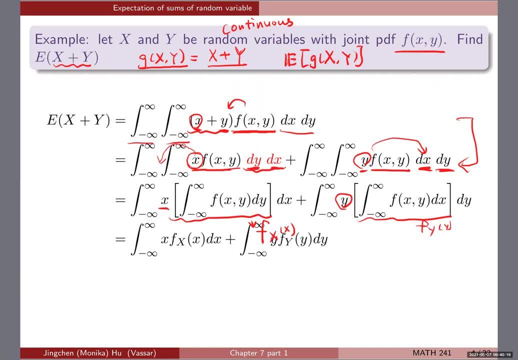 what we're going to do for the next step. okay, let me um try to erase maybe this part. okay, uh, but you know what i mean, right? so here we are getting um, the integral, the inner integral, becomes a marginal density, marginal pdf, and then we're going to get the marginal of y over here. okay, so, 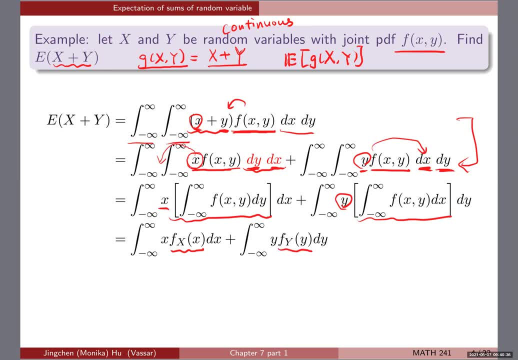 this is the marginal density of y over here. okay, and then, lastly, if we look at this term, this is our old friend. okay, we're doing integral of x times fx, okay, dx, okay, so what, that is. that's the expectation of x. okay, similarly, we get here. the second term is the expectation of y. 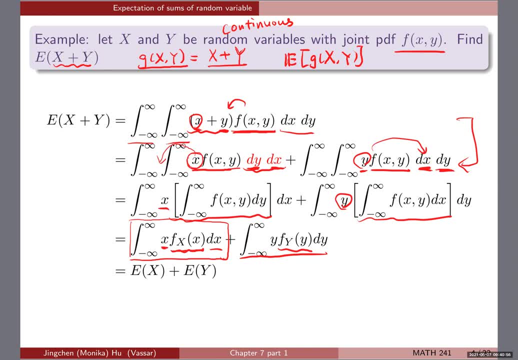 so this goes down to um expectation of x plus expectation of y. okay, so what this is telling us? okay, this example is actually a very important result. okay, and this is also the title of this section- expectation of sums of random variables- and what this is saying is that, if i know the joint pdf, okay, of x and y, the expectation of x. 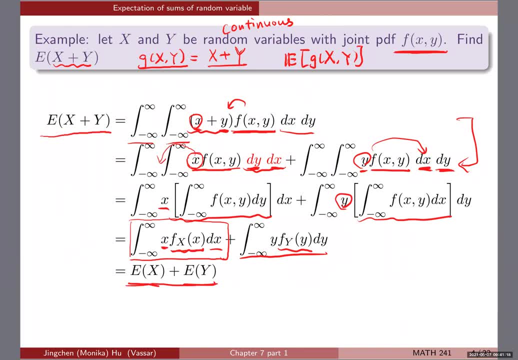 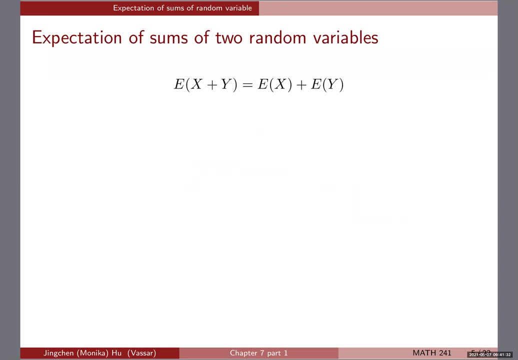 plus y is the sum of the two expectations. okay, so in this slide we show how you can arrive there, okay, and then some of the techniques i think are really important to to grasp, especially about those integral, um, double integral integrals. okay, so this is a general result, like i said, okay, and then um. i would just also mention that we showed 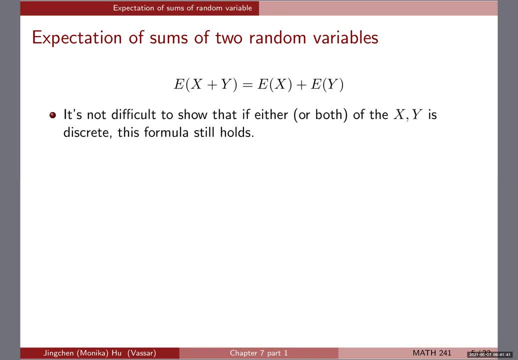 the case for the continuous okay pdf, okay, uh, continuous random variables. but if you also tried it to work it out with discrete case, you will work as well. either one of them is discrete or both of them and another thing is, uh. this result does not require x and y to be independent. 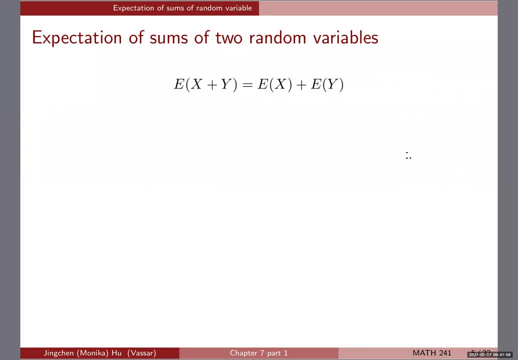 okay. so if you come back to, uh, what we showed earlier on this, uh, slide of proof, okay, nowhere we assume anything about independency and we also assume that the individual Mr and Mr x are respective, and so you can get it right if you actually want to know what the individual Mr and Mr x are different. 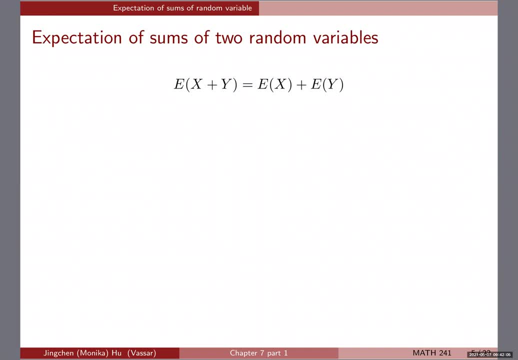 okay, so we can get it right. if you actually want to know what the individual, Mr and Mr x are different, Okay, And so, as you can see, in this case we don't need them to be independent. you can always apply this result. Okay, Moreover, it can be generalized to n random variables. Okay, so here I'm writing: x1, x2 through xn. Okay, so the expectation of the sum of them is the sum of all of the expectation of each of them individually. Okay, 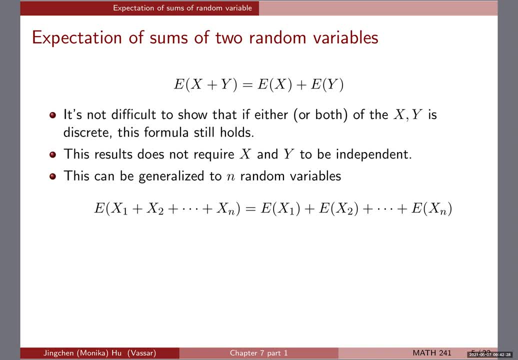 Okay, so that's a really important general result and we should be able to use it in many cases. Okay, but I also wanted to bring your attention to another function of x- y, which is the product. Okay, so remember, we're working. the general result that we have of the joint function over here is: you find the expectation right is the g, x, y function, and then we have that general result at the beginning to show the expectation of this function. 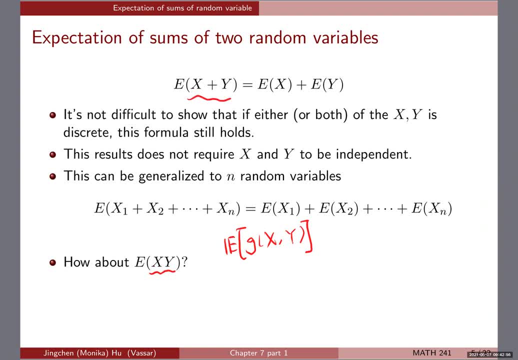 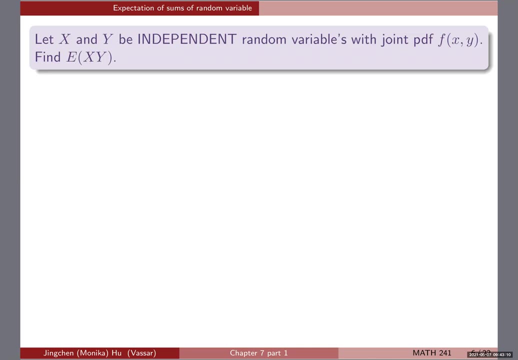 Okay, so earlier this is the x plus y is the g x y function. Now, x times y is the g x y function. Okay, so we have a special case here to show you. Okay, and then we're going to also highlight the implications here. Okay, so the exercise or example here is: let x and y be independent. Okay, they're independent random variables. Okay, they have a joint PDF. f, x, y. Okay, you are asked to find the expectation of x, y, x times y. Okay, Alrighty, so we're going to start. 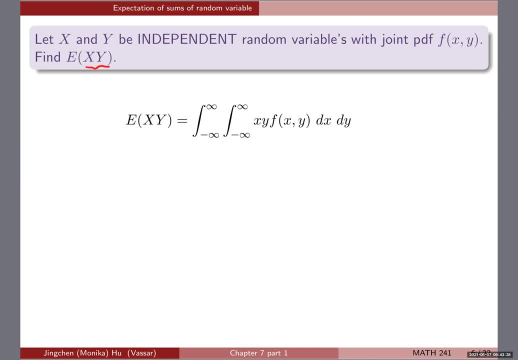 one by one. Okay. so, remember, our g x y function now is x times y, So we put x y over there, Okay, and then it's f x y, which is the joint PDF that we have, And then right now I'm putting down just dx dy. we're going to see whether we're going to do this or maybe switch the order, Okay. so the next step. Okay, remember, we have a extra condition here. Okay, we're also like not only just any kind of x and y. we know that they're independent. 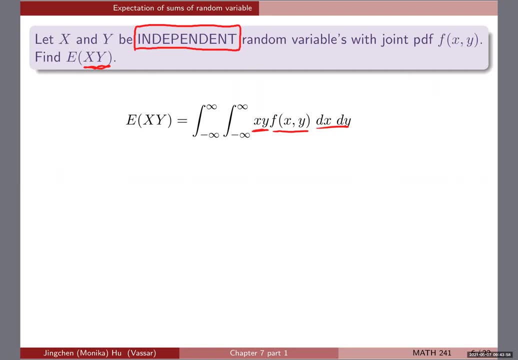 from each other, And because of that, a very important next step that we can take is to break this joint f x, y into the product right of the marginal, And that's what we know. If you remember, if two random variables are independent, if they're continuous, then their joint PDF is the product of the two marginals. Okay, it goes the same for for the discrete case as well, But since here we're working with continuous random variables, so we're going to do that one here. Okay, so that gives us to the second step. 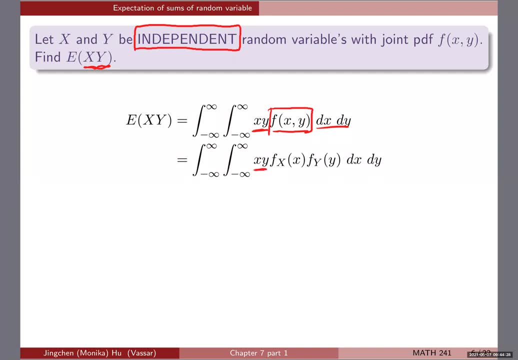 Here. so we still keep our x- y here, Okay, And our joint f x- y becomes f x times f y- Okay, and then dx- dy, Okay, All right. So now, if we go to the next step, we're going to use something very similar to what we did with the x plus y case, That is, if I'm doing the inner integral of dx first, then anything not about x is a constant right And meaning that we can bring it outside of the integral. 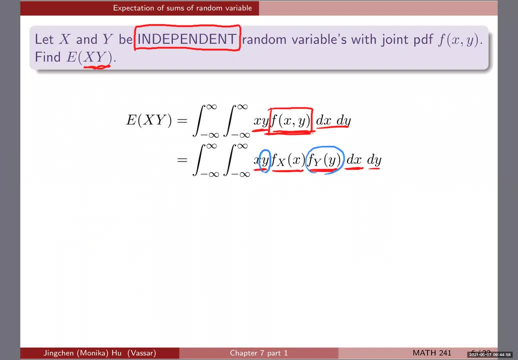 So y is a constant, Okay, f, y is another constant, Okay, so I can bring both of them outside. That will be a really handy thing to do. So let's see: Okay, so we brought it out, Okay, And so they're here. And then the inner one. Now, you remember, right, we just saw it. this is the expectation of x, Okay, So what this does is that, well, we realize that one part of this is one part of the double integral is is the expectation of x. 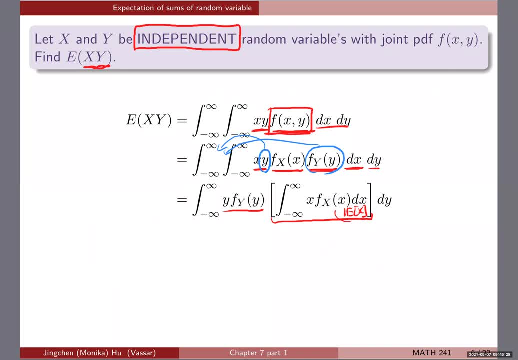 Okay. And once we write it out as an expectation, this e, x, okay, becomes a constant right with respect to y. So we can further bring that out from the outer integral as well, So meaning that we can bring this outside, Okay. so what that does is we have expectation times, the single integral, and this single integral, as we know, is the expectation of y, Okay. so that's why, finally, if x and y are independent, notice that it's very important to have this condition, because if they're not, 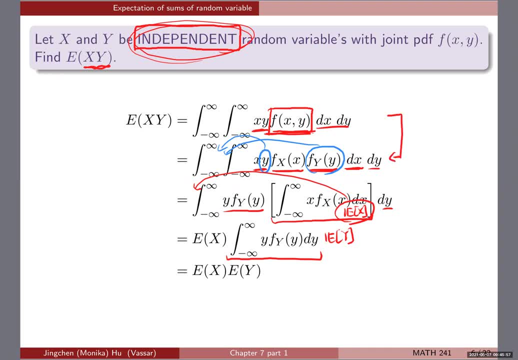 independent, they're not going to be independent. If they're not independent, we cannot even go from here to here. Okay, this, this line one to line two, is due to independence, Okay, And so what this result is telling us is that if x and y are independent and you have their joint PDF, then the expectation of the product is the product of the expectation. Okay, so a couple of notes here. The first one is like what we were saying earlier: this formula only holds when they're independent. Okay, But also, this is not a sufficient 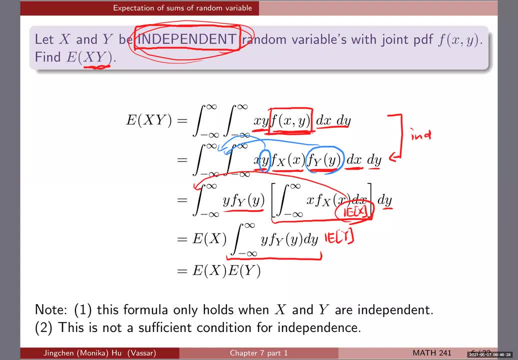 condition for independence. Okay, meaning that sometimes you might have like expectation of x plus times y indeed becomes okay, the product of the, the expectations, but that doesn't say that they're independent. Okay, the condition, the sufficient condition for independence, if you remember, is that their joint PDF can be broken down into the product of the marginal PDFs or, like the joint CDF right can be broken down into product of the joint PDF. 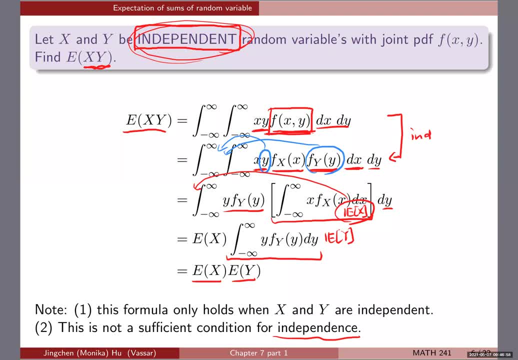 Okay, and those are for the continuous case. if you're working with a discrete case, then it's about the PMF, Okay. so what this is saying is that, well, if you know that they're independent, this result holds. Okay. But if you have x and y particularly satisfying this result, it does not guarantee that they're independent. Okay, But anyway, usually right, like what this exercise is doing- you're given that they're independent, So so you know this result and then that will be really handy to use. Okay, But if you're